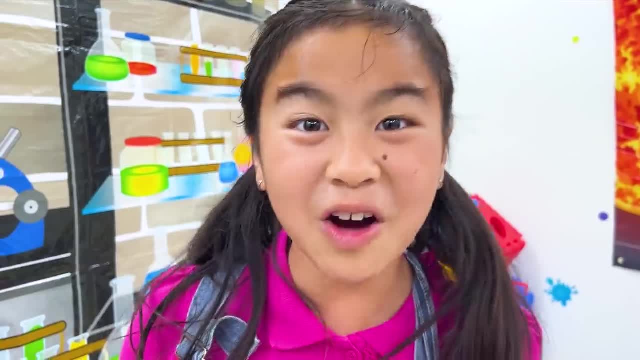 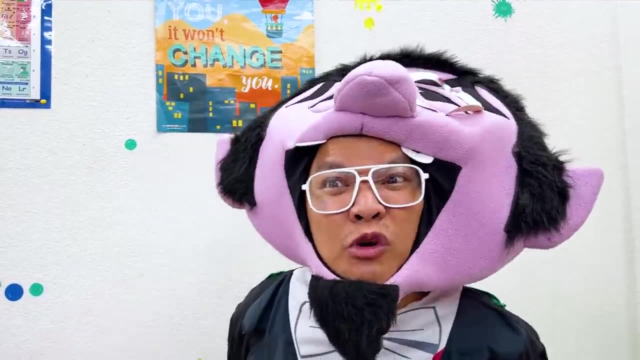 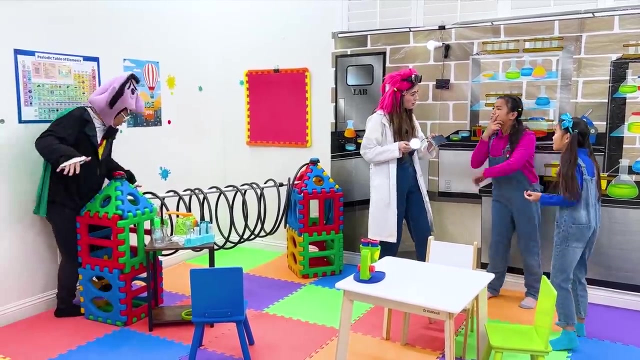 That's not interesting. Whoa, that's so interesting. Wow, My magic doesn't work with solar energy. I'll be right back. Do you know where solar energy comes from? This stuff, Chiropractic, Yay, Yay. 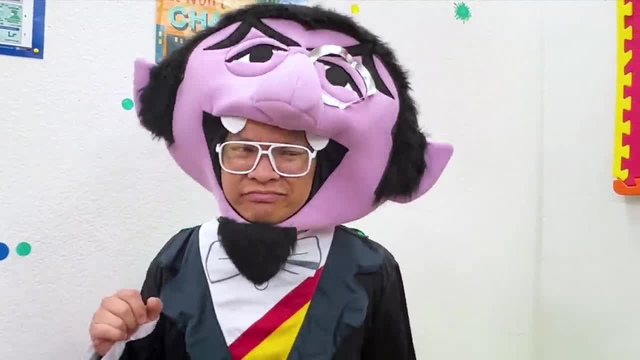 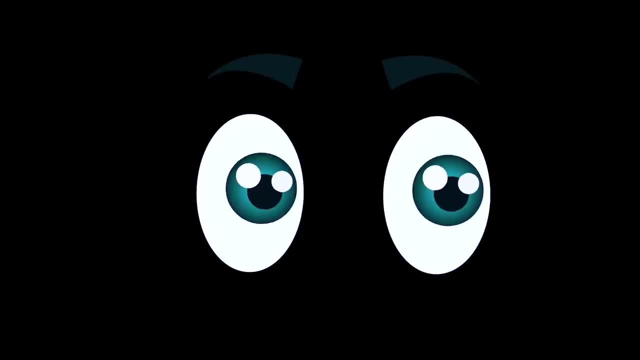 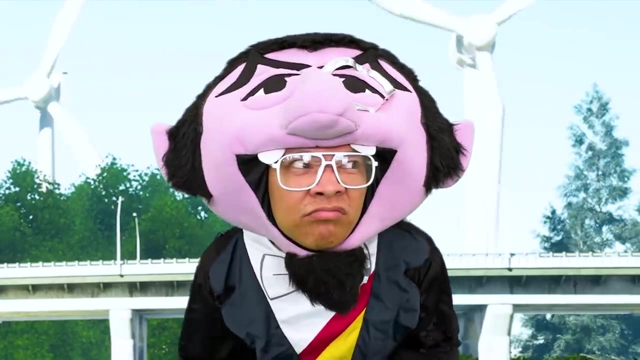 Solar energy, The sun, Huh, The light is out again. Auntie, I got this. Huh, Where are we? We are in the land of wind power. What? Where is this place? Oh, the giant turbine. 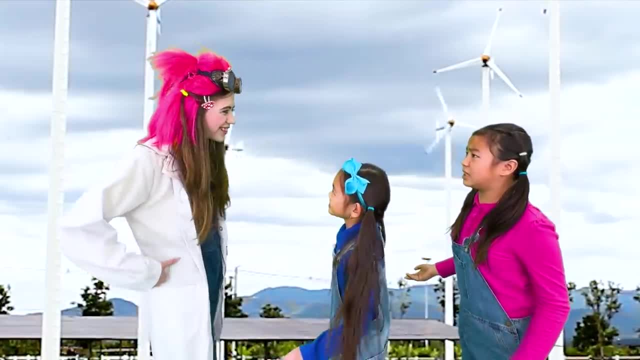 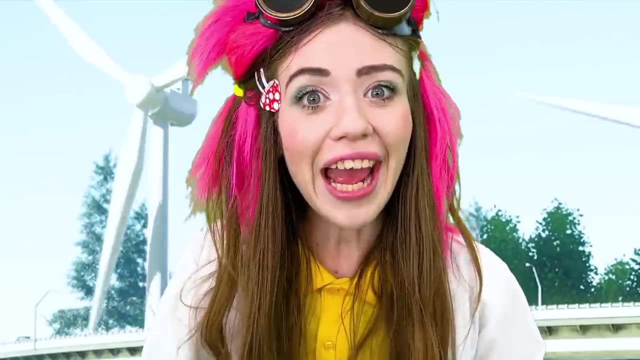 Wow. Well, what are they for, Auntie? The wind helps the turbine spin around and generate energy. Wow, But I still don't understand clearly. That's okay, Let's go back and I'll explain to you, Huh. 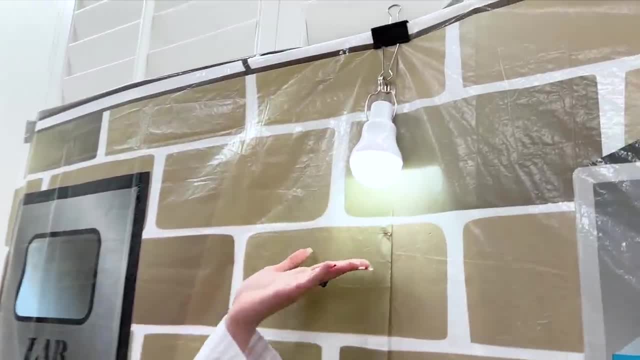 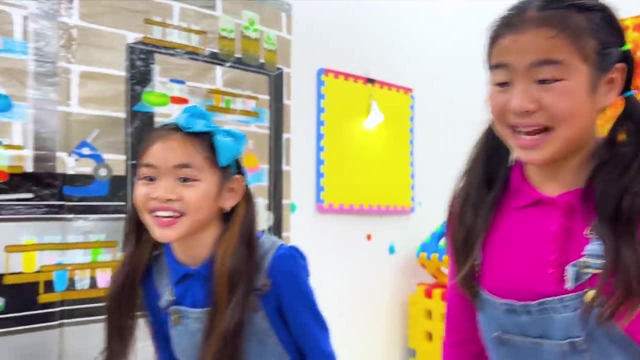 Why is the wind? right again, Because the wind collected energy, which lights up these bulbs. Here's another one: Whoa More light. What is this Auntie? This is a model of a wind turbine like we went to before. 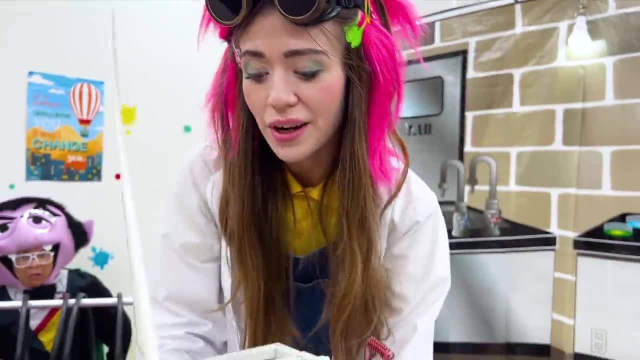 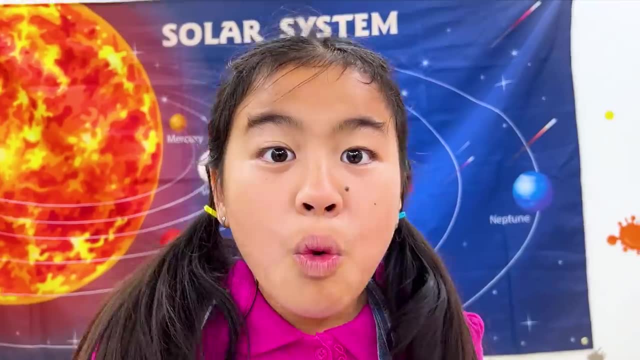 Awesome. How does it work? As the wind spins the turbine, it generates electricity. If you look over here, you can see the light. Cool, Wow, That's amazing. That's not that amazing, Ooh, so cool. Magic doesn't work with wind energy. 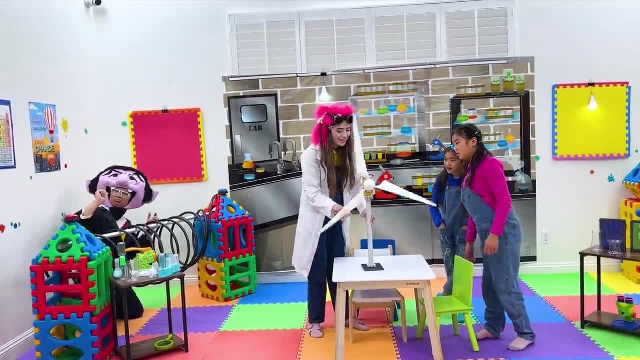 Kinetic energy is the energy of motion. As it moves, it generates energy, which is electricity. Wow, Now I understand. There's no point in understanding that. Huh, The lights went out again. Auntie, Yeah, I got it. 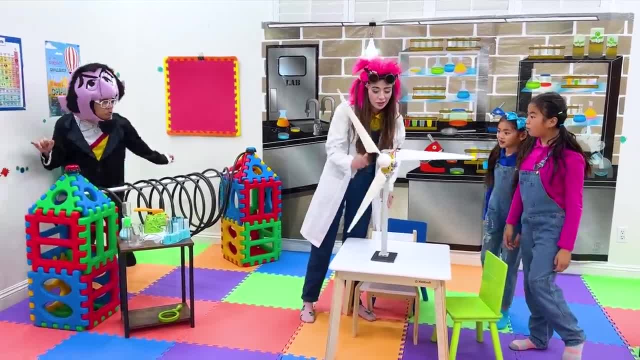 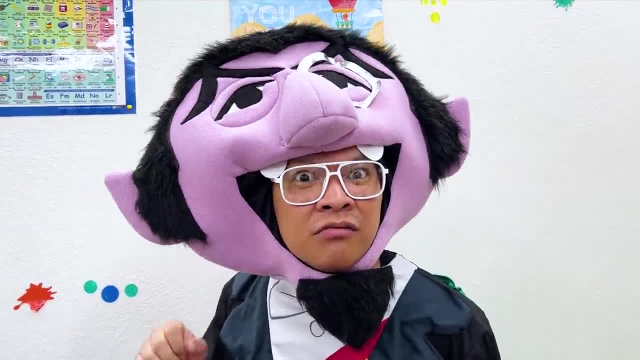 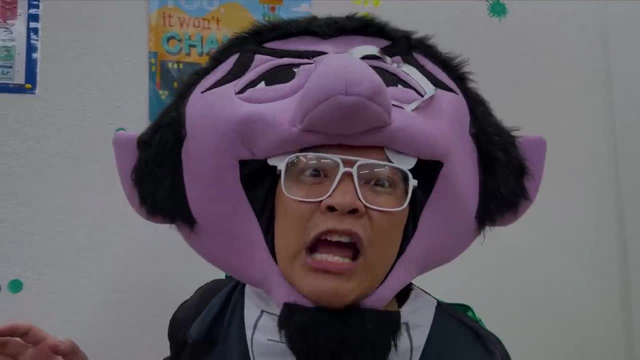 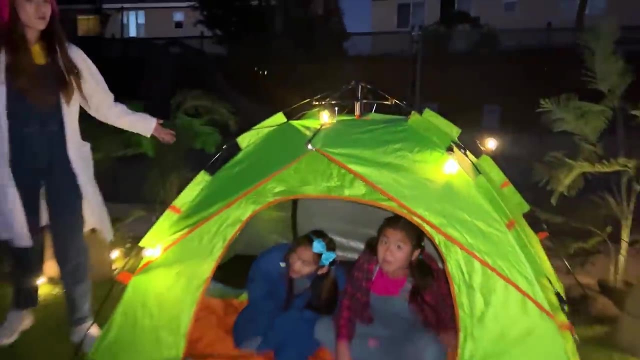